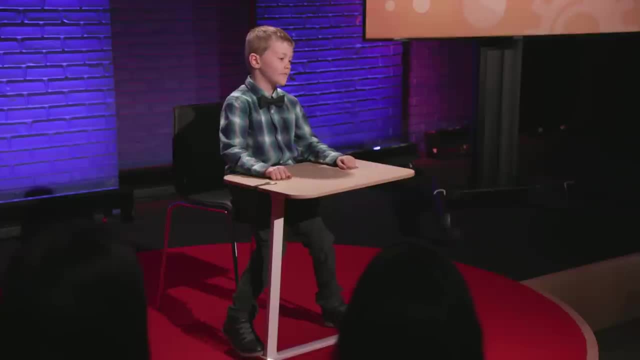 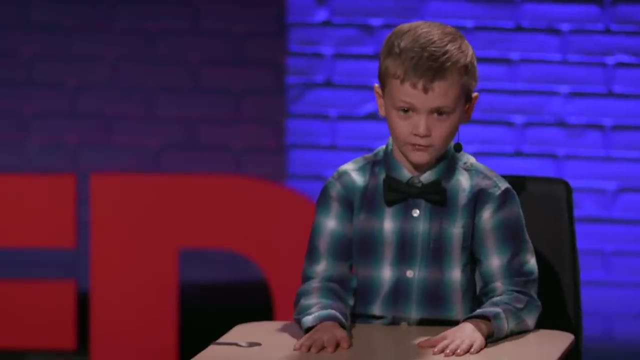 myself math as a toddler. I'm even writing my own book about adding, subtracting, multiplying, dividing and negative numbers. I'm also going to have lots of equations in my book. Math is everywhere: When you buy things, drive a car, pay bills, hold time. 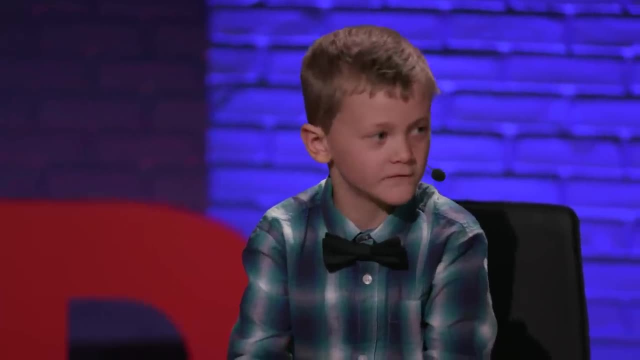 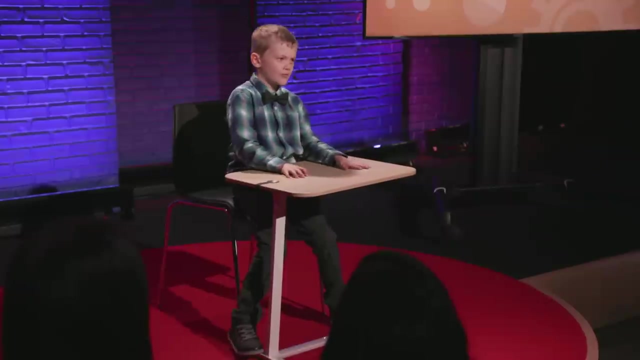 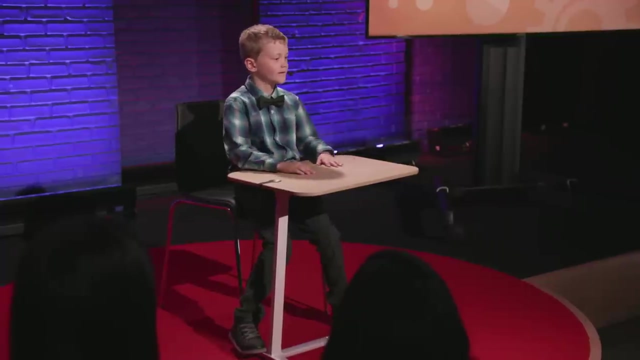 anything when you're cooking. multiplication is used by a lot of different people. did you know? we even use multiplication to tell time on a clock. it works like this: if the small hands on the seven, that means it's seven o'clock, smaller hands on the eight, that means it's 7, 40. i use multiplication. 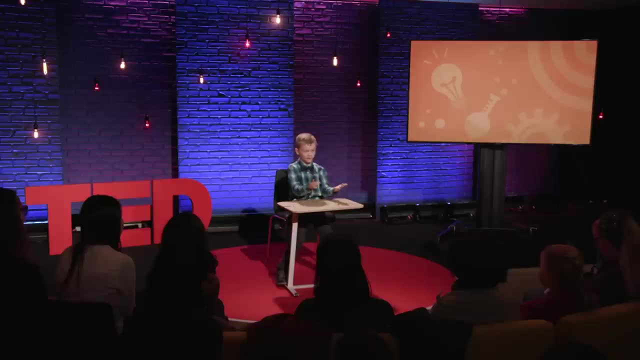 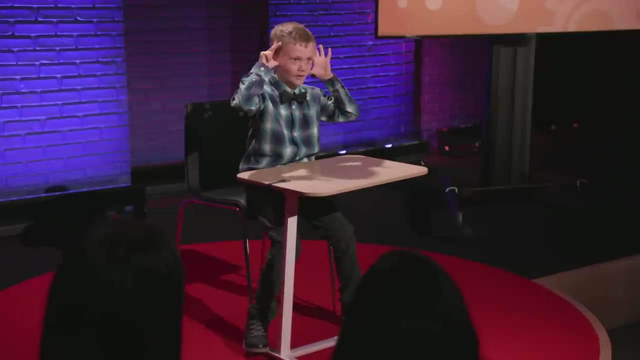 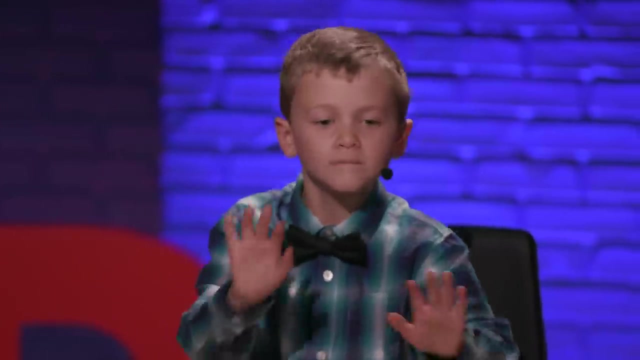 5, 10, 15, 20, 25, 30, 35, 40.. 40 5 times 8 equals 40.. the clock says to 740.. i learned how to tell time because i kept getting frustrated not knowing how much time i had to play before bedtime. 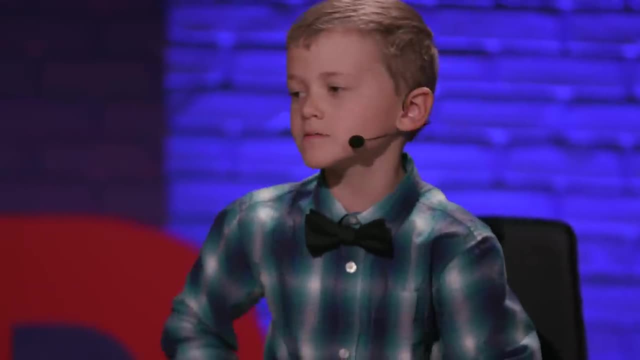 but if i have to go to bed at 8 And the clock says it's 74 d and i can calculate how much time i have left, in this case i will say the time is 15, 15, 10, 15, 20, 25, 30, 35, 40, 50. 15 times a day equals. five times 5 times 8 equals 40. my clock says it's 7: 40,. I learned how to tell time because i kept getting frustrated, not knowing how much time I had to play before bedtime. But if I have to go to bed at 8, and the clock says it's 740, then i can calculate how much time I have left. In this case, i want to guess. In this case I've already said I was going to count abt 9 and So rarely, And of course, no On the table. 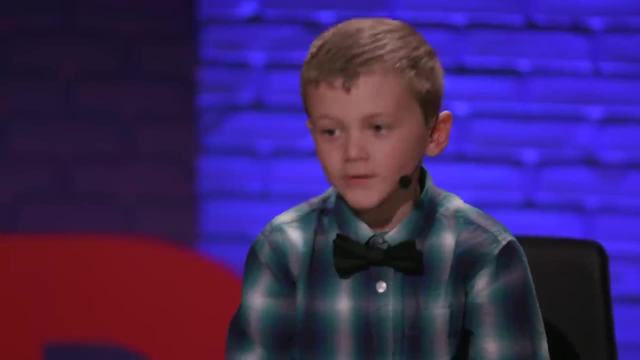 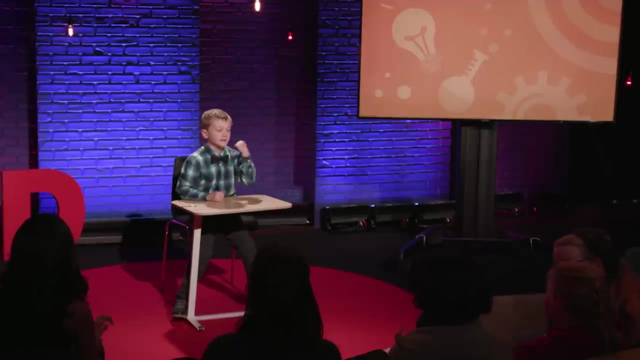 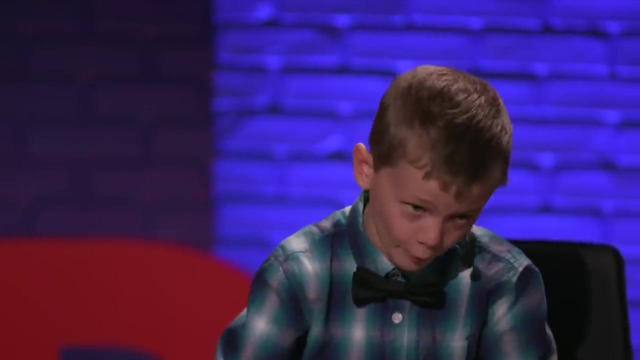 a whole twenty more minutes to play. First graders use multiplication too. For example, you can tell how many kids can be in a classroom. Just multiply how many kids at a table by how many tables there are. Audition notes are very important too, and can be very important. 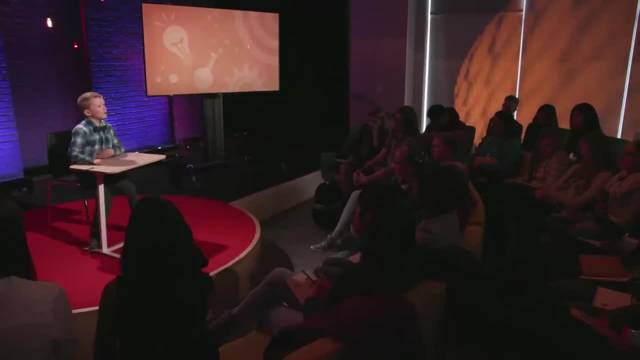 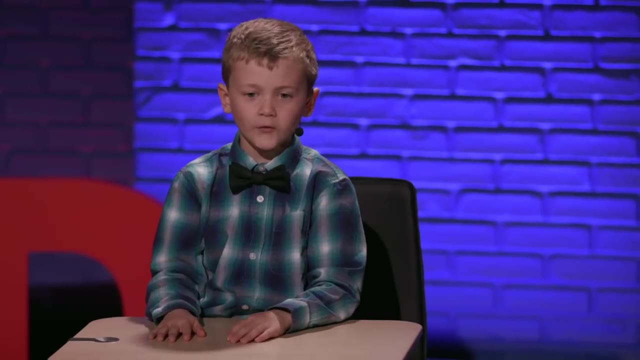 For example, let's say you're ordering cookies for all the kids at the party with the principal. You definitely want to make sure you have enough. So if there are thirty students already at the party and one hundred seventy more students join the party, how many cookies? 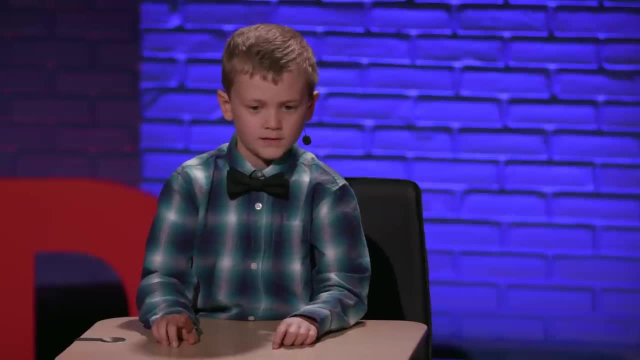 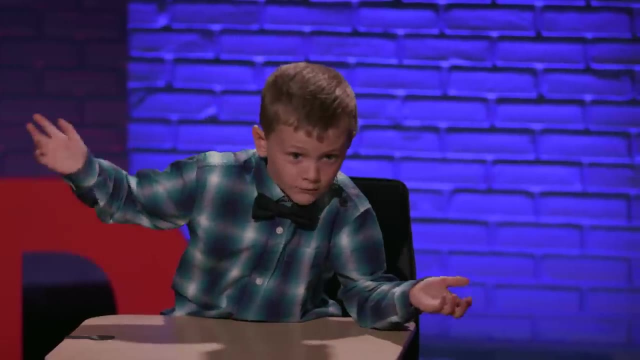 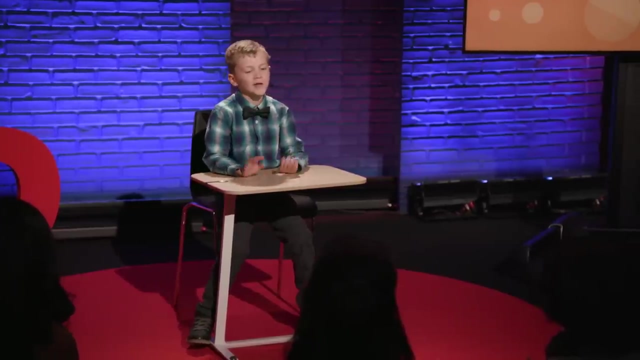 do we need now? Wait? Let's say we invite the rest of the school and a thousand more students joins. How many cookies do we need now? 1,800.. Also said 1,200.. Another example is in science. Let's say I need ten potions.